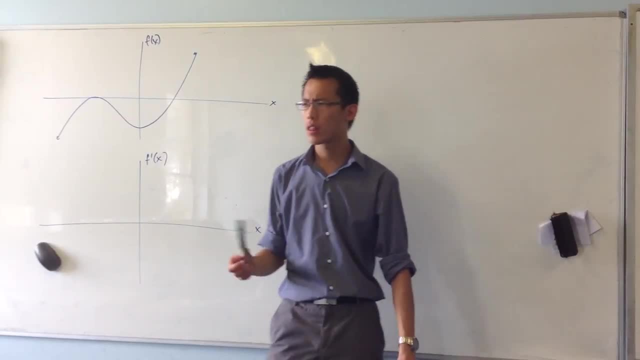 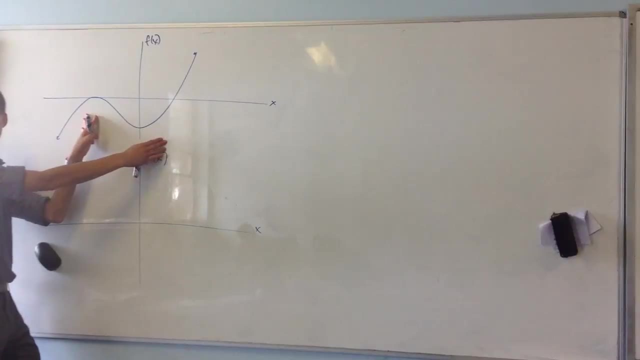 So, going from f to f, dash, just differentiating ones. What are the most important features? okay? Well, we're going to mainly look for stationary points, right, Because anywhere there's a stationary point here. what does that tell you about the first derivative? 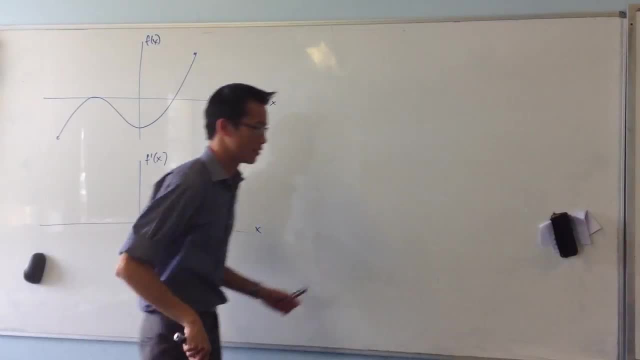 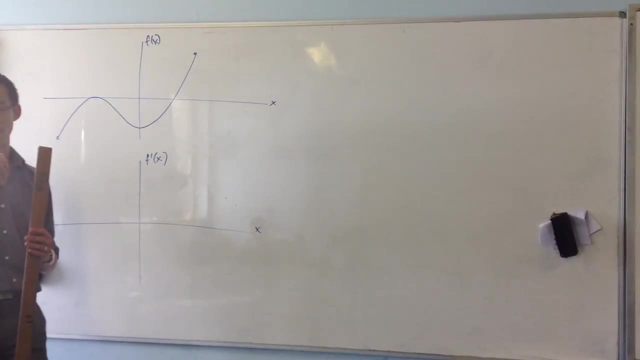 Should be zero, right? good, So I would get. do I have a ruler? Here we go. I'll get my ruler out, okay, And sometimes they'll actually give you an extra sheet of paper on the end of the exam and you'll have this on it. another thing: they'll say: attach including your answers, right? 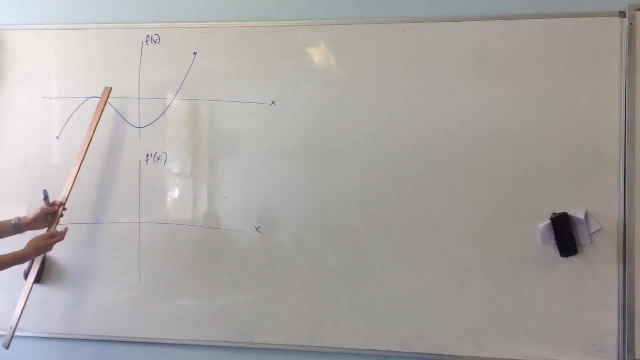 But they're quite far apart. So that's what the rule is for. yeah, All right. so with my other color, let's see how well this works. You'll line up to your stationary points, Okay, and you draw it down. 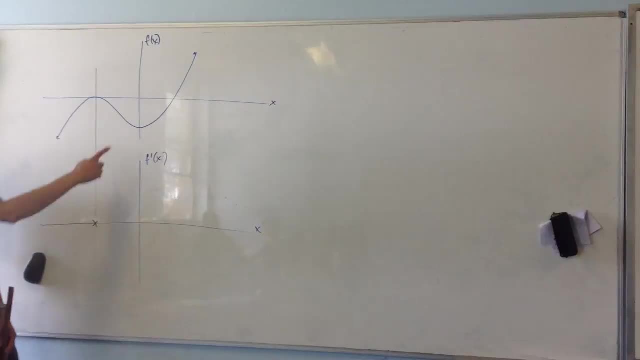 So now you know your first derivative is going to land there, okay, And you repeat the process for the other stationary point. But, as you can see, this is actually on the axis, so I don't need to draw another line there. Here we go, okay. 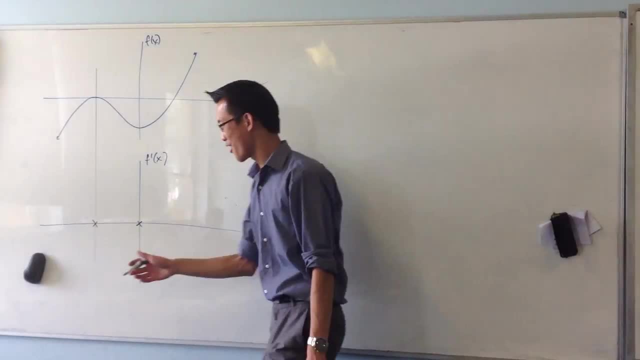 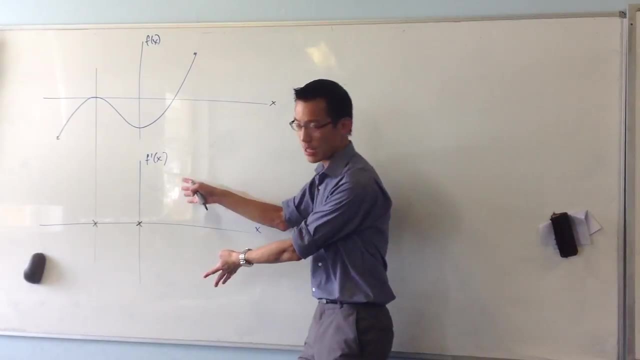 All right, now don't get confused at this point. Now that I know I've got this, I've got these two points where it's zero, okay, I need to know what it does in between those places. yeah, So derivative, the gradient function tells you that is this increasing or decreasing right? 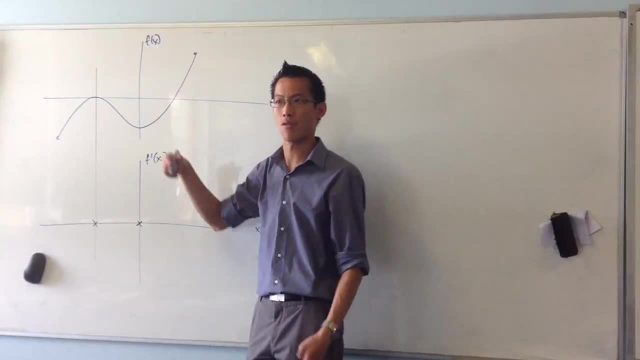 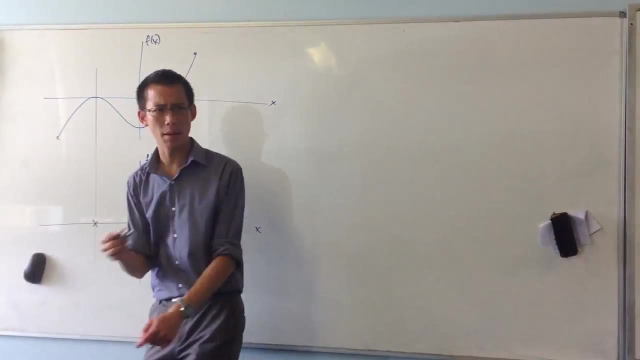 So on the graph of F, I'm going to label whether I'm increasing or decreasing. okay, So let's look at the left of this stationary point: Am I increasing or decreasing? Increasing- And sometimes you'll see it signified with plus signs like this: 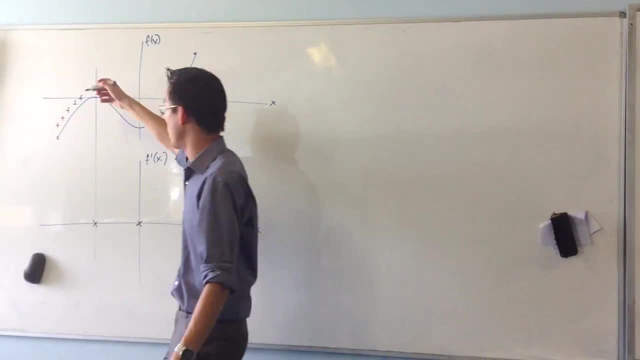 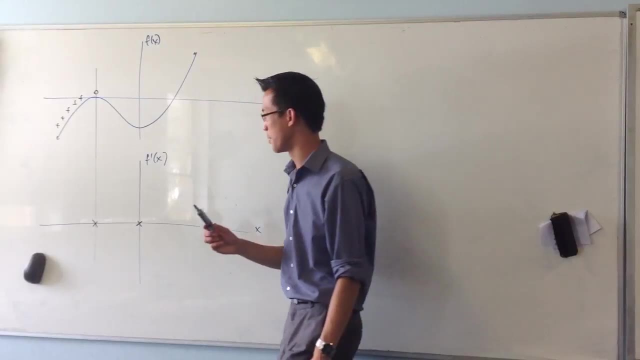 Okay, so I'm increasing, And then at the stationary point I'm not increasing anymore. okay, So that's why it's zero. So that means that if you kind of see, I'm out of colors- I usually use green for this, but since my gradient should be positive here, 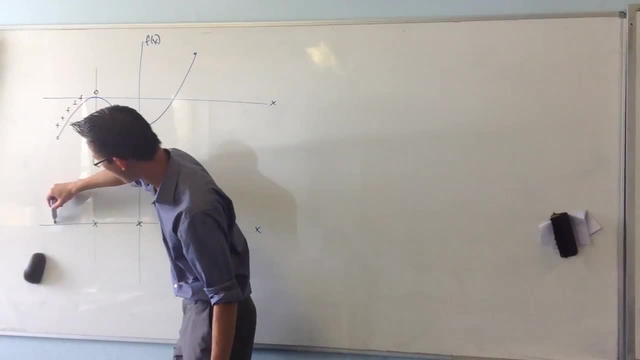 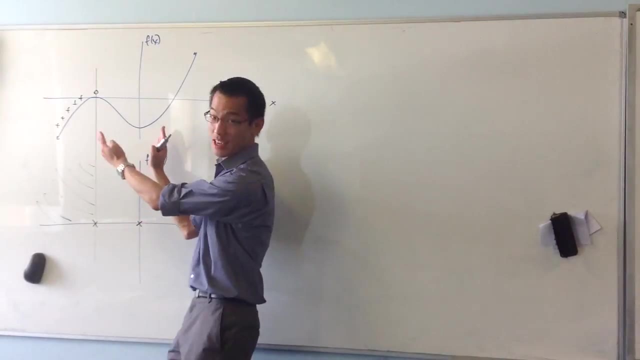 when I come down to this graph, I ought to be above the axis. I ought to be drawing somewhere up here. Hopefully that's light enough not to interfere. okay, All right. in the same way, what am I doing between the stationary points? 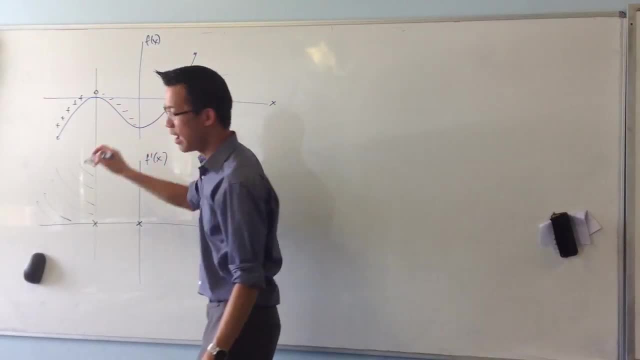 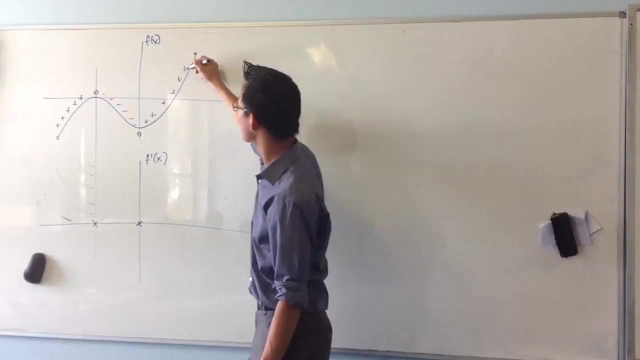 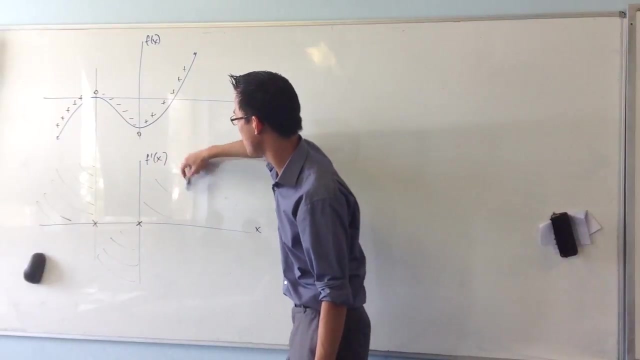 Decreasing, And you can see usually if it's a turning point it's going to, you know, flip the other way. Okay, So I'm going from positive to negative, back up to positive again, And now I just have to sketch something that's going to go. 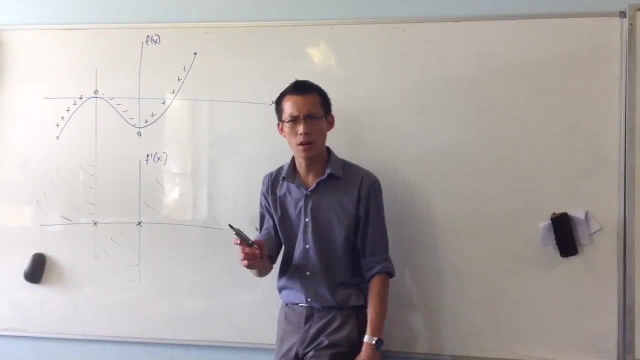 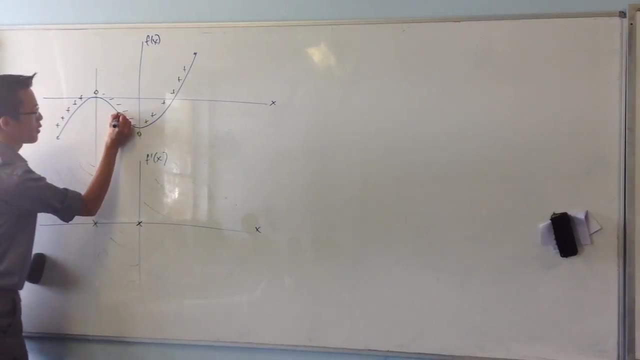 through those regions and satisfy that. okay, Now I should be careful as well. There's one more feature that I've missed off the graph of F that I haven't taken notice of. Yes, That's right. So since there's a point of inflection here, what's that going to mean for F dash? 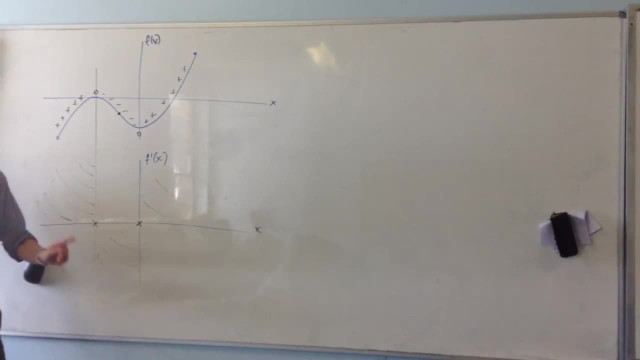 That should be a stationary point down here. okay, Just got to be careful with your language, because stationary point here doesn't mean stationary point here, right? So just watch out for some of those. So this again, I'm going to get my ruler out. 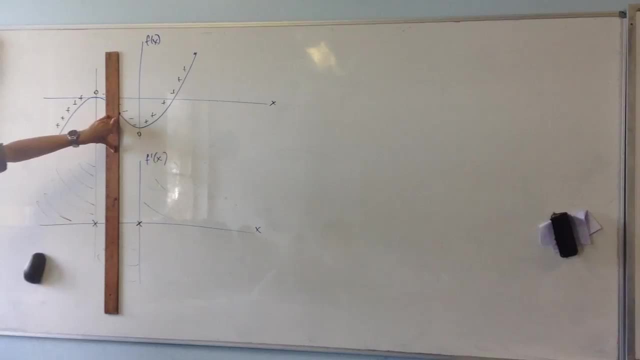 Typically what you get- I mean what I've drawn- is a cubic right, So you're generally lucky with those. The point of inflection will be symmetrical. There's going to be symmetry between the two turning points, So draw that down. 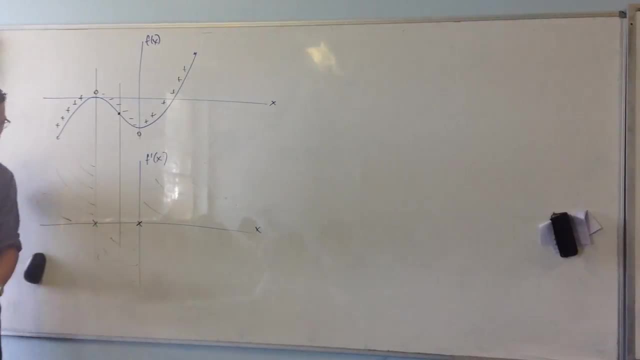 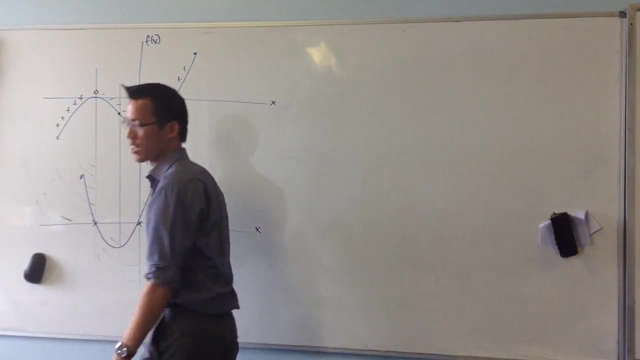 It ought to be halfway, okay. So I'm going to get my stationary point for the first derivative there, okay, And that's it Now. we just draw a line that will fit like so And I'm done. Where it starts to get trickier is if you ever get asymptotes involved. 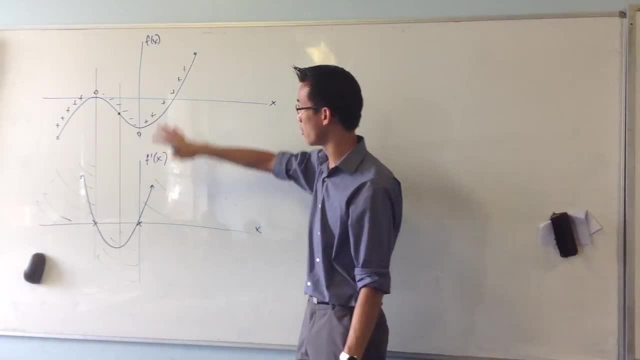 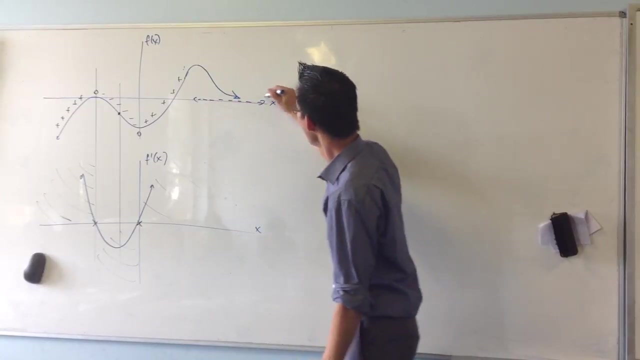 that kind of thing. if you've got a vertical or a horizontal asymptote- sorry, a horizontal or oblique asymptote up here, okay, Let's just suppose. Let's suppose it did this. Let's add another stationary point And suppose it approached y equals zero, okay. 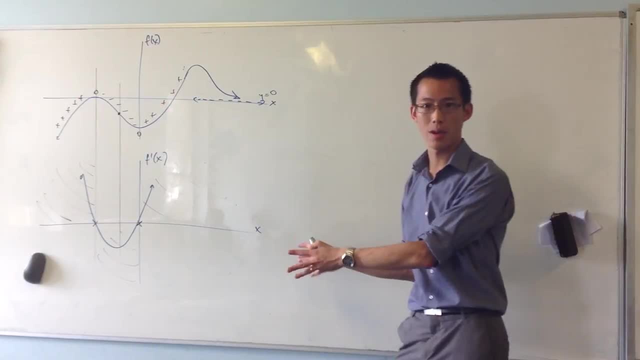 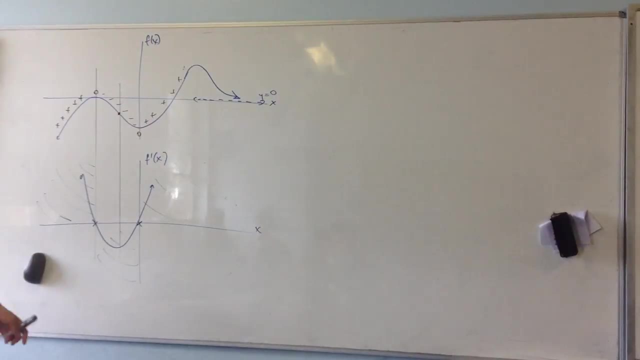 So everything else is not changed. okay, What am I going to add to this graph to make it reflect this? What should I do? Okay, good, So the first thing, I've added a new stationary point. okay, So you always think about big features first, like stationary points. 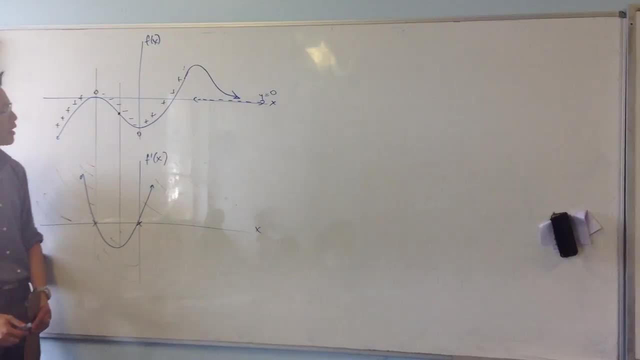 and then you add little features in, like the inflection point afterwards. okay. So, like we said, I'm going to add a new stationary point. okay, So, I'm going to add a new stationary point. okay, So, I'm going to add a new stationary point, okay. 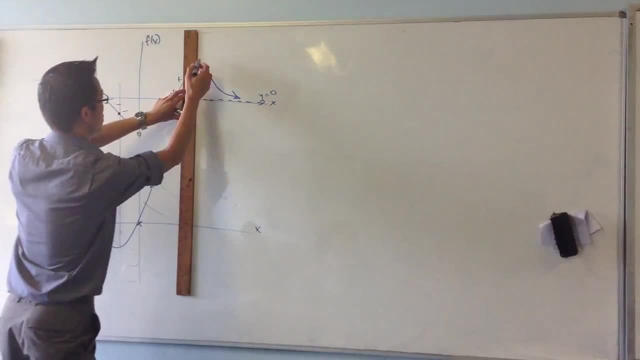 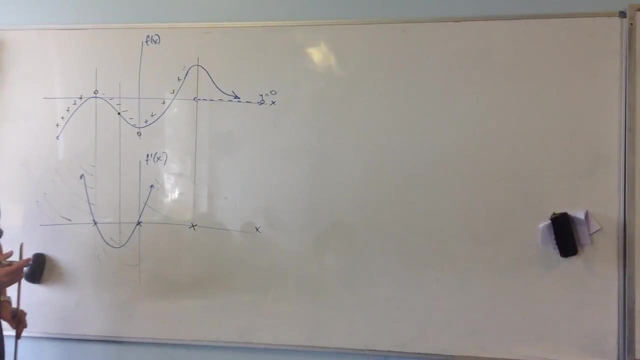 So, like we said, we just added a stationary point. okay, So that means that at this point here it's going to go zero. okay, Now it's positive, positive, zero, negative, negative, negative, negative, negative. 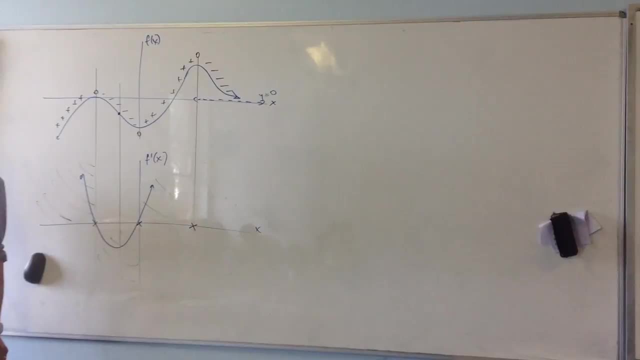 But it's not just any negative, is it? It's a point of inflection, Okay, so, yep, there's a point of inflection somewhere around here, Like I don't know roughly, let's see, That still looks concave down to me, right. 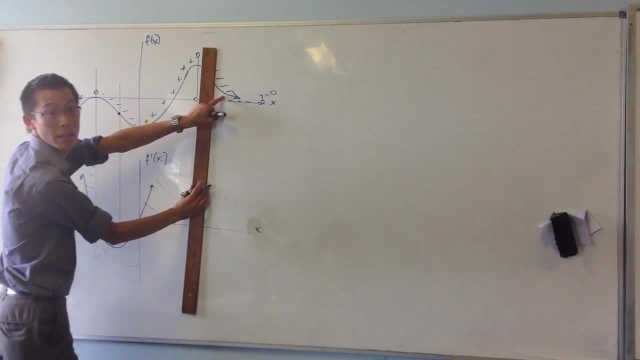 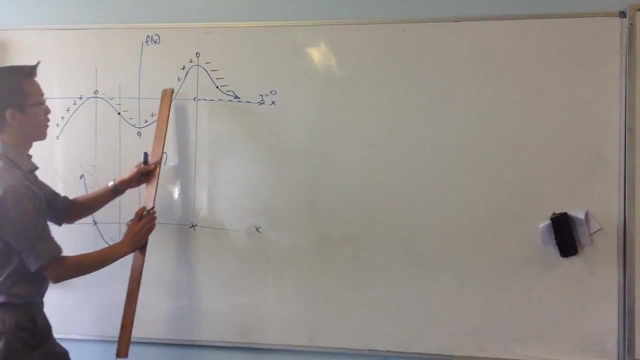 And then somewhere around here it just looks concave. It changes the concave up, yeah, So it's quite subtle, So I'm going to call it there, okay. So that means that on this graph I'm going to have a stationary point. 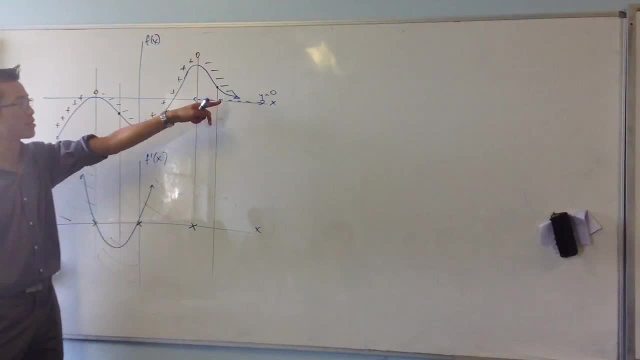 Okay, Now one last thing, As this approaches infinity, as x approaches infinity, what is the gradient approach? Minus zero, Minus zero, Zero from the minus sign Right. okay, So it is going to be a negative. 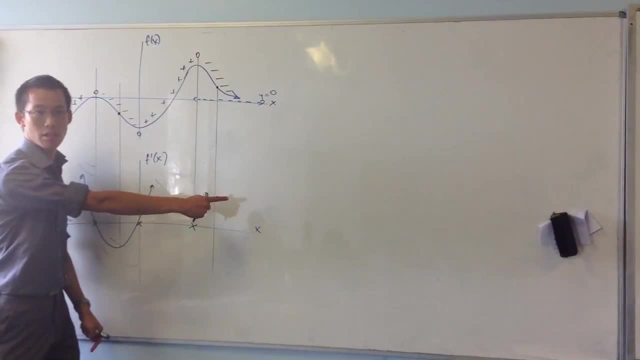 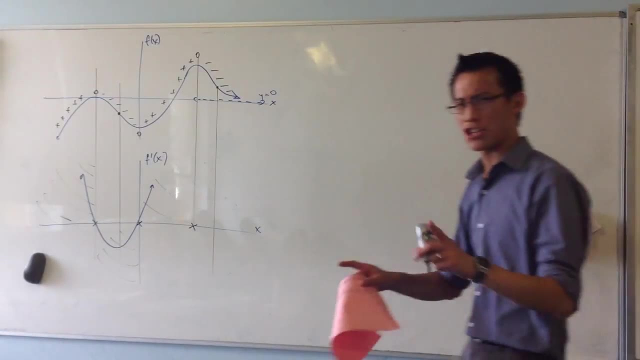 It's going to be a negative number because I'm decreasing all the way, right, But I should be getting closer to the axis, okay, Right, So did you catch that? My gradient's approaching zero? Yes, Is that okay? 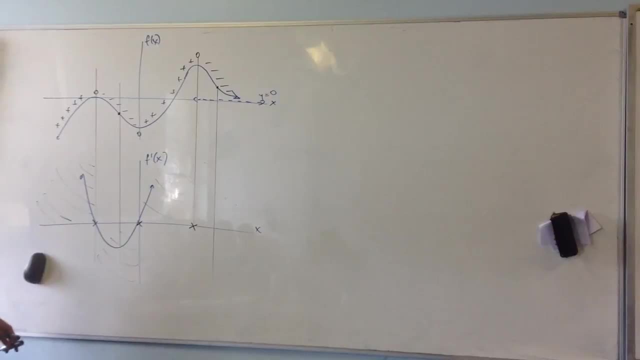 So what's going to happen here? All right, I've missed the point of inflection, haven't I? Yeah, because you're thinking: how is this going to come back down? So I don't know, let's just put it there, but you get the idea. 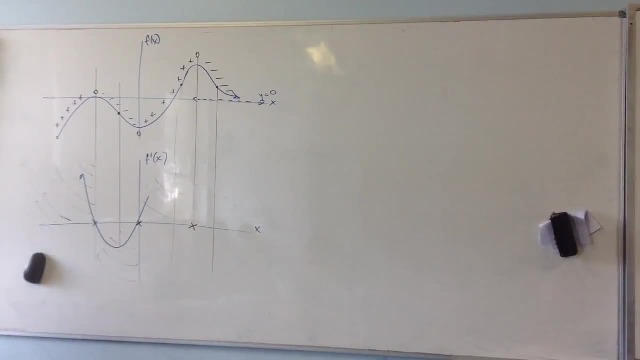 Okay. So what's going to happen Instead of that kind of thing? what's going to happen Instead of that kind of shape? it's going to come up, but then it's going to slow down. Here we go. So that's the point at which it's steepest, okay. 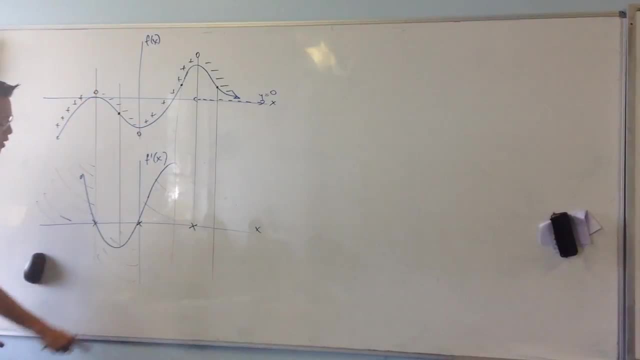 So that's why that's the point where the gradient is highest. yeah, Okay, I've got to come all the way back down here. There we go. There's my stationary point. I'm going to turn around again. another point of inflection. 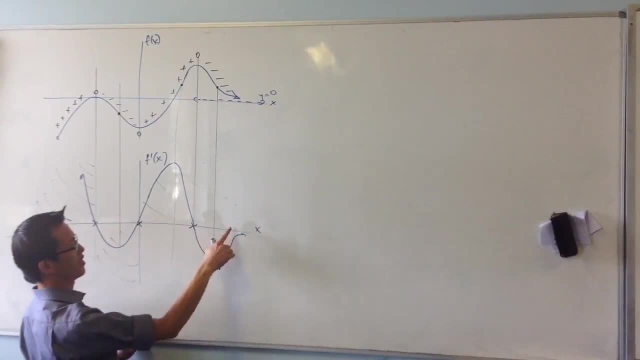 Now what happens? I've got to approach zero. Oh, this is really wonky. sorry, It's because my axis is bad. Okay, so in this case, f is approaching zero and f dash is also approaching zero. Can you think of a situation where f dash would not approach zero? 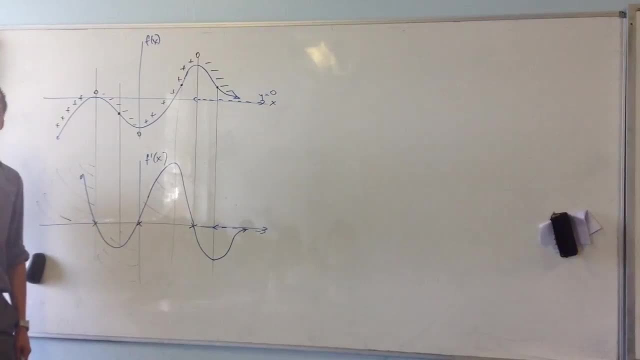 Yeah, It would approach a number if it's approaching a b-casson term which is a straight line. Good, okay, Yeah, that's right, It would approach a b-casson term if it was approaching a b-casson term which was a square function. 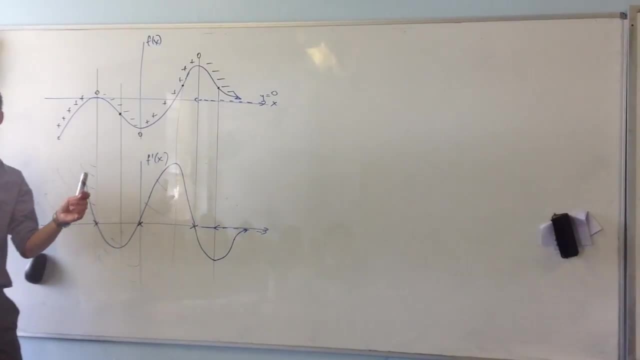 That's right. Okay, so all the functions you get here. here's the idea, right? If you didn't catch that, why am I approaching zero here? Well, when you differentiate a random zero, you're getting zero, okay.